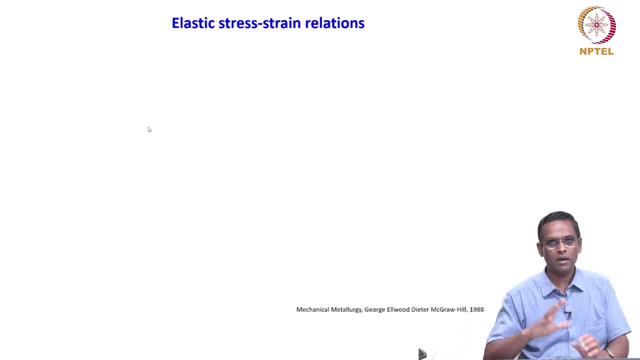 Okay. So we have spent considerable time on the description of the stress and description of the strain and some important, I would say, the properties of the stress. So we are going to go through this, Okay, Okay. So we have seen all these tensors and their parameters Right Now. we will slowly get. 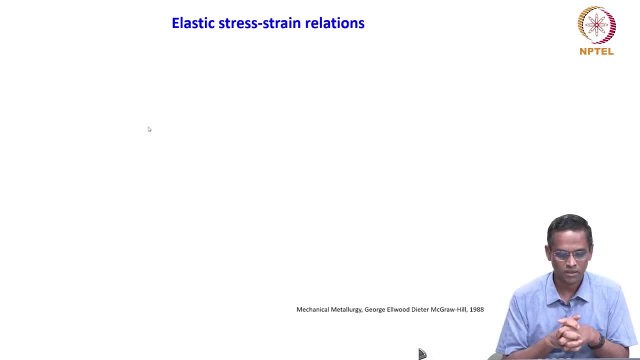 into relations between stress, elastic stress and elastic strain. Please remember we are looking at only small strains and which is purely elastics, Right? So when we say elastic deformation, then it can be compression as well as tension. So you take these two. 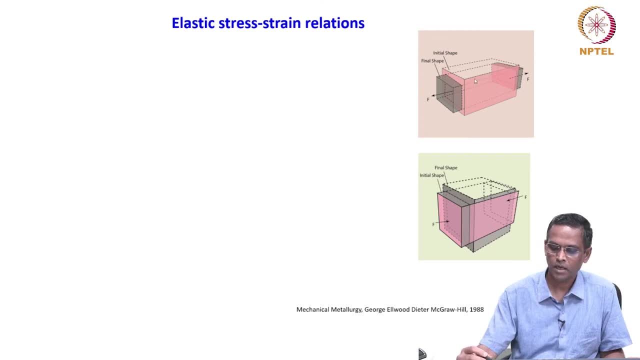 So you take these two examples. This is an initial shape of the member body and which is being subjected to tensile deformation. That means the length increases, the width decreases. Similarly, this member is subjected to compression, then the length decreases. 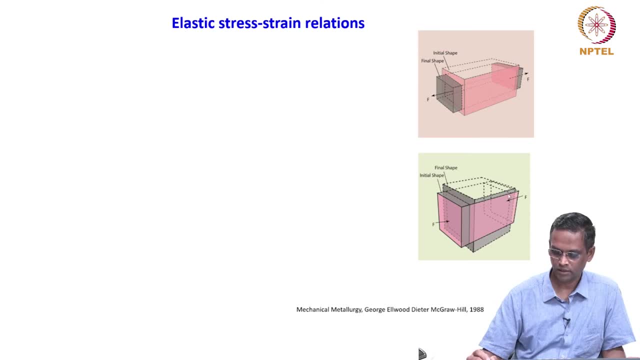 the height increases. Okay, The height increases. So that is something normally we expect. This is in a pure elastic deformation. So if you want to relate a stress tensor to the strain tensor, we must introduce material properties. The equation of this nature are called constitutive equations. 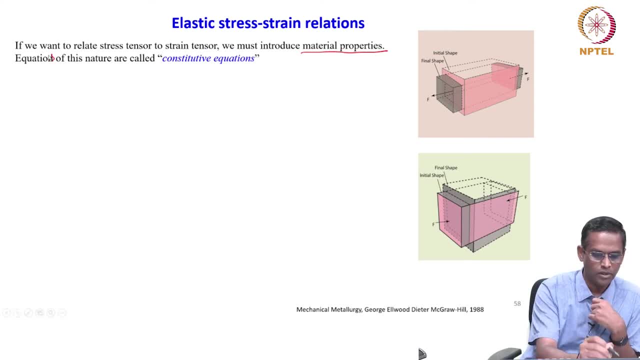 Okay, So what is this constitution equation we are familiar with? This is a well-known Hooke's law: Sigma X is equal to E times Xn, So this is a linear elastic deformation. So this is a linear elastic deformation. 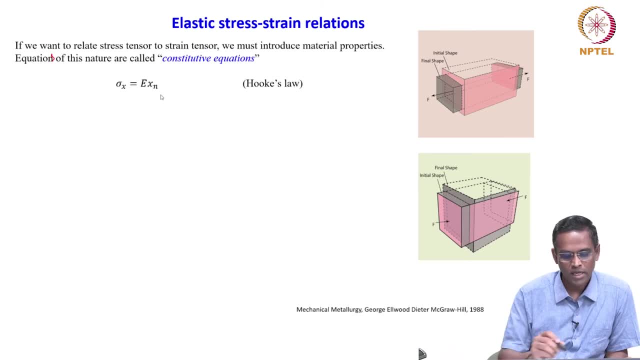 Okay, So E is the material property which is modulus of elasticity in tension or compression in a linear fashion. So the transfer strain has been found by experience to be a constant fraction of the strain in the longitudinal direction. This is known as Poisson's ratio. 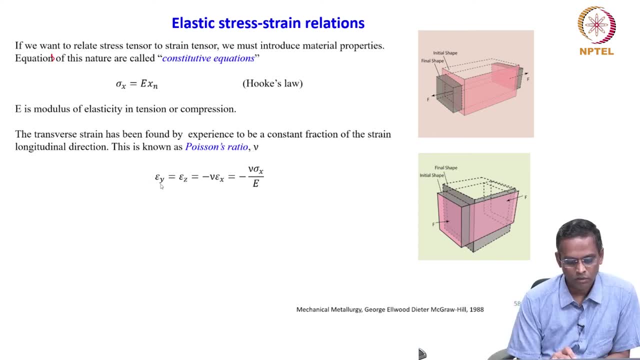 Okay, So this means you can express this: epsilon Y is equal to epsilon Z is equal to minus mu times epsilon X, Right? Or it can be related to the stress, which is also can be related to minus mu. The epsilon X can be written as sigma X by E, Right? So this is a simple. 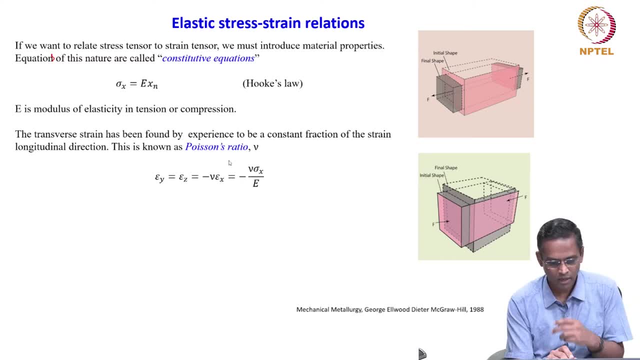 so this is a simple relation. First time we are writing a relation between a strain versus stress in a linear. For most metal, mu is 0.33.. So this is for a single dimension. So if you are interested in developing this relation for the 3D state of stress, you have to complete the 5 battery. 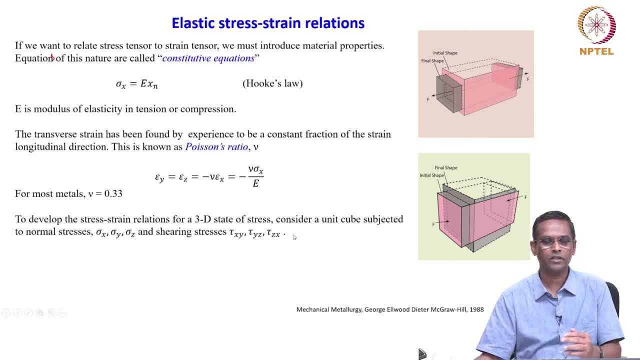 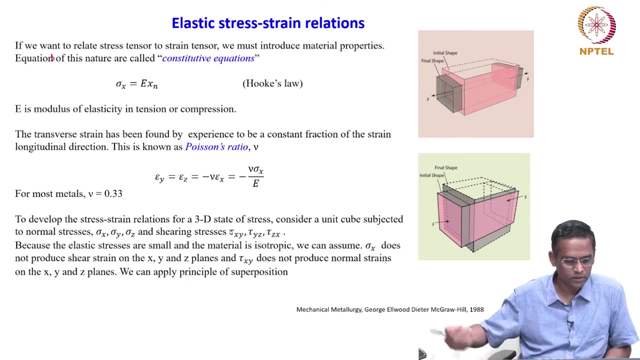 stress. and then we should consider a similar cube where we have just looked at for description of a stress at a point, similar geometry. you can imagine where all the normal stresses, sigma x, sigma y and sigma z, and shear stresses were marked okay. So, and before we get into the relation of the stress strain in a 3D state of stress, 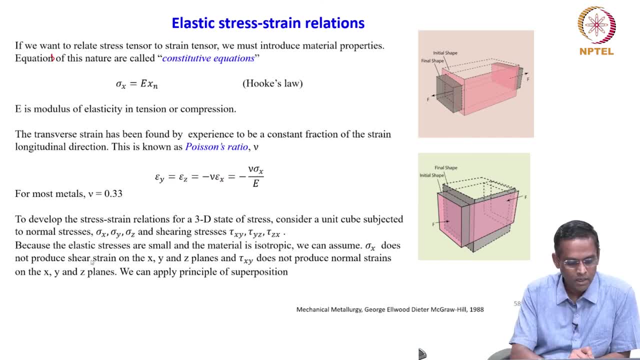 there are some assumptions. What are the assumptions? Because the elastic stresses are small and the material is isotropic, very important, right, you have to pay attention to these details. If these are the conditions, if the material is isotropic and the elastic stresses, 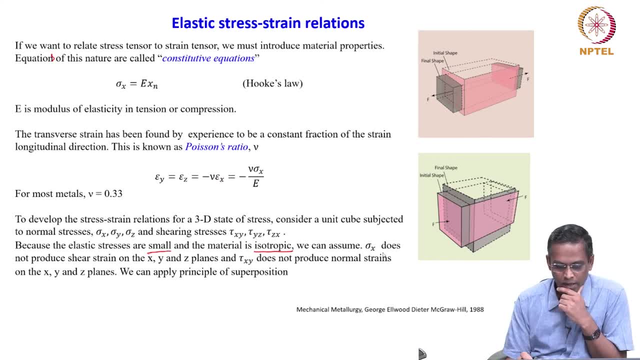 are small, then the material is isotropic and the elastic stresses are small. right, If the material is isotropic and the elastic stresses are small, then we can assume sigma x does not produce a shear strain on the x, y and z planes and tau x- y does not produce. 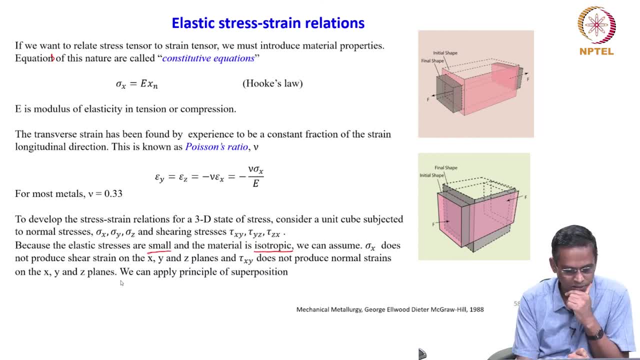 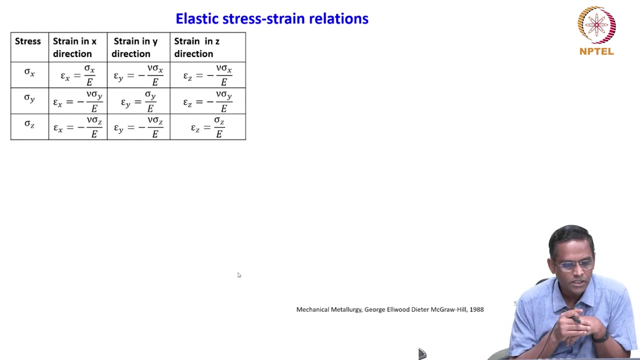 normal strains on x, y and z planes, We can apply principle of superposition. So under this conditions, the sigma x will not have influence on superposition. Then we can use a principle of superposition. So what is that? So this is. this is a table. 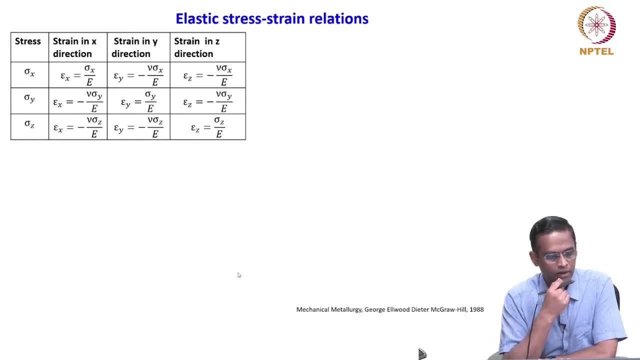 3 by 3 matrix. you can create using similar what we have just written there For a stress in x direction, sigma x. we can write a strain in x directions epsilon x is, which is sigma x by e, But the strain in y direction can be written epsilon y is equal. 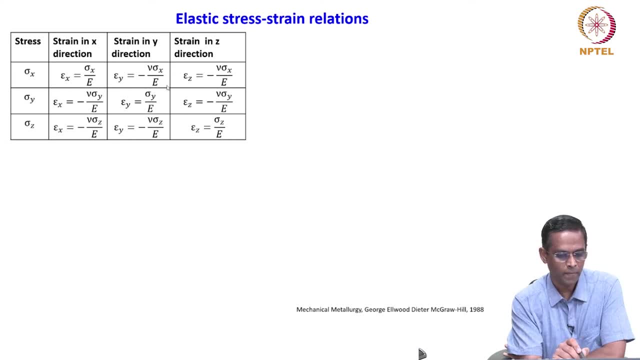 to minus mu times sigma x by e. This is epsilon. z is equal to minus mu sigma x by e. So what does it mean? We are now looking at the effect of stress in the x direction, but what its effect on or what kind of strain it will produce in. 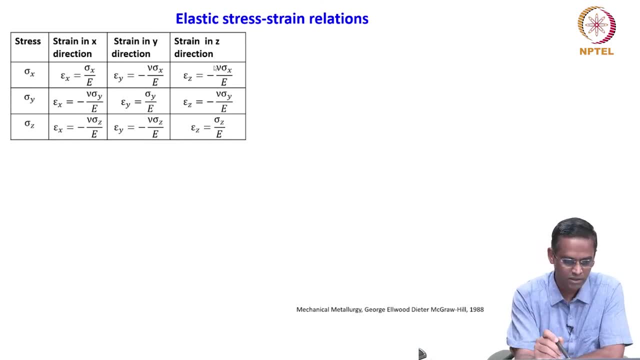 y direction and z direction can be expressed with the simple relation. That is what you have to look at it, okay. Similarly, you look at the strain. the stress is x normal stress, that is sigma y is a normal stress in y direction. 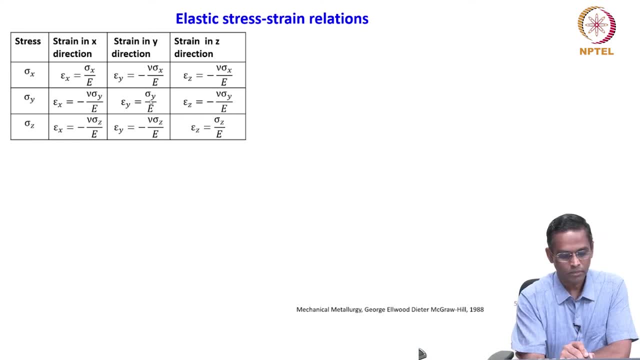 So this is a normal stress. So this is a normal stress. So this strain in y direction is simply given by sigma y, by e, But the effect of this on x direction, that is, if you want to see what kind of epsilon x it will produce, or what. 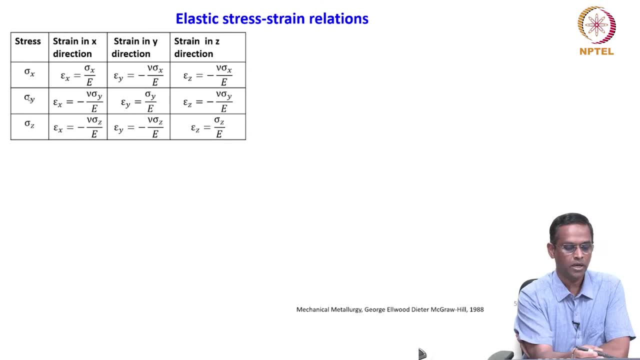 kind of epsilon z it will produce, just by the normal stress which is acting in y direction. then we get this kind of relation. So that is So. this is the beauty of this superposition of the strain components in the x, y, z directions. 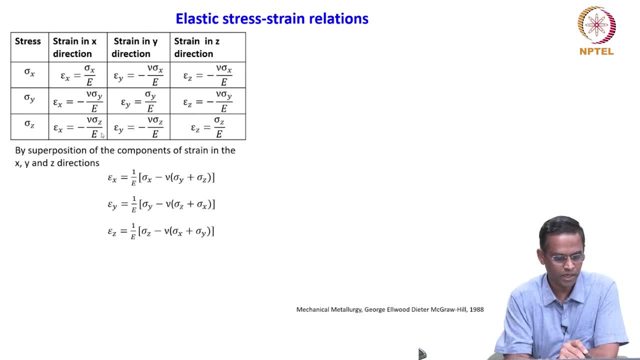 So we can just simply write like this. So, whatever I have just put in the table, you can just write it like this: epsilon x is equal to 1 by e, sigma x minus mu. Okay, So you can write. you can write this at any interval of time: sigma y plus sigma z, right? 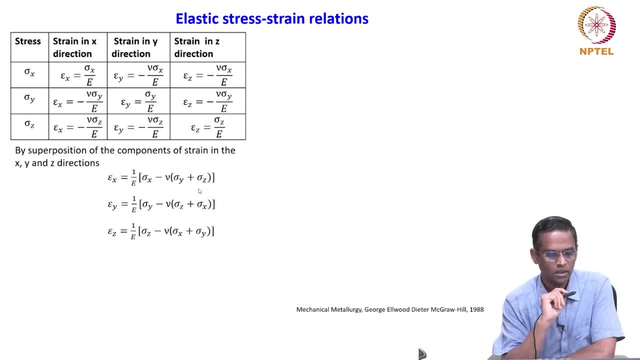 So that is what it is. So. so these kinds of relations can be written for three axis. So this is called a generalized Hooke s law. right, This is called a generalized Hooke s law, It is. that means stress, strain relation in three dimension. 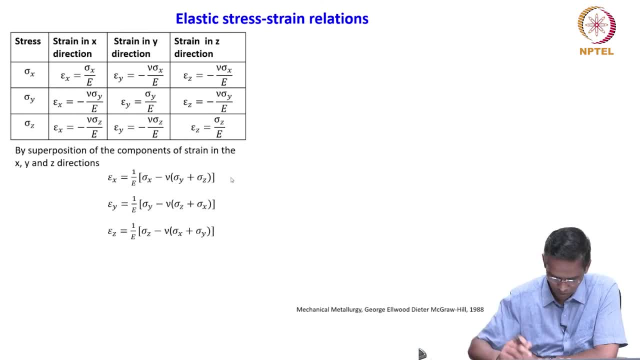 So I will show a few examples of this. The first example is that this is called a generalized Hooke's law. That means the stress strain relation in three dimension. So that means sigma y plus sigma z. So the shearing stresses acting on the cube produce, that is, tau xy, is equal to g times. 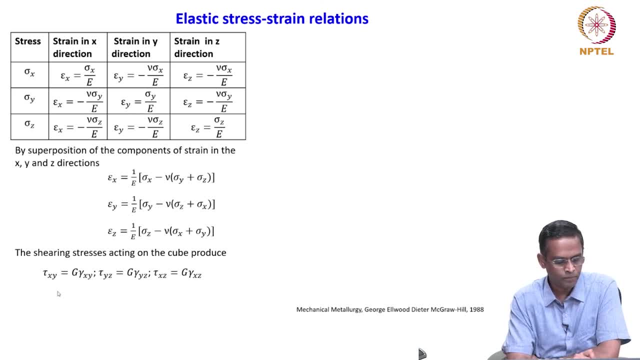 gamma, xy, shear stress and shear strain, and this is g is a shear modulus, Similarly in yz and xz and directions. So you have three constants now: E, Young's modulus, g, shear modulus, mu's Poisson's ratio. These are the constants involved in the stress strain relations for isotropic. 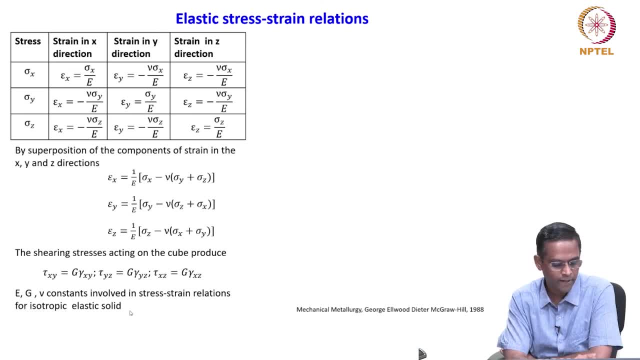 elastic solids. Please understand, this is very important. These relationships are fully valid for isotropic elastic solids. And then we can now look at the other relationship where this elastic constants have Another constant, volumetric modulus of elasticity. what is that? So, which is k? So sigma m is mean stress. we know sigma m by: 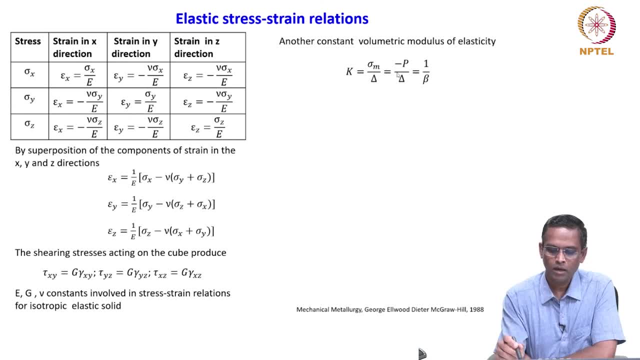 delta, delta also, we know, which is also equal to minus p by delta, which is equal to 1 by beta. What is this? Where minus p is a hydrostatic pressure and beta is the compressibility. So these are some general relations these stress strain components have. 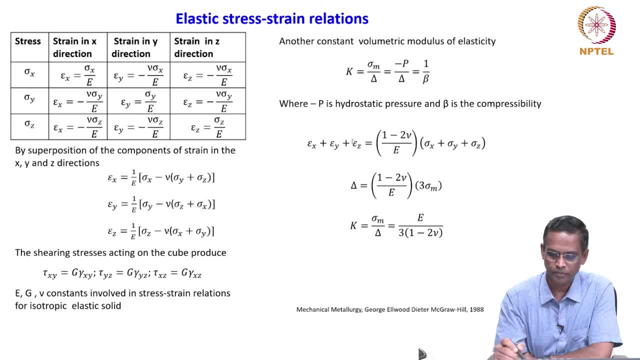 So we can just try to put this into perspective, how we can write this Again. another relationship you have, k can be related like this: and then, and basically what we are trying to see is we are giving, trying to give another relation for volumetric modulus, which can also be written like this: k is equal to 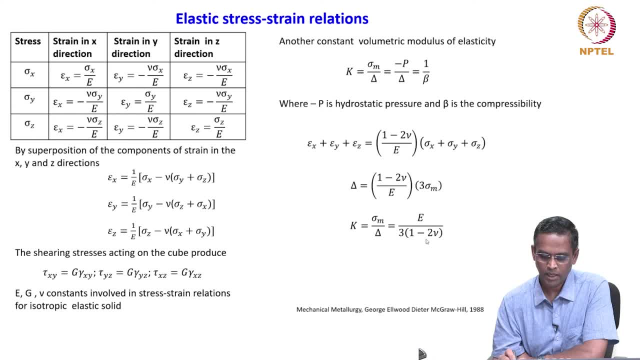 sigma m by delta is equal to E by 3 times 1 minus 2 E. So all these relations will be handy if you try to solve some, some small problems in the area of elasticity. We will try to use it when it comes especially. 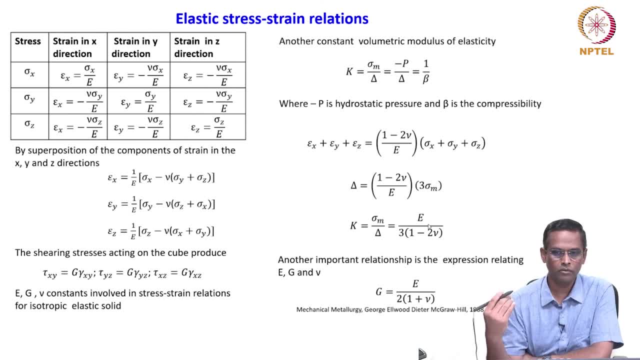 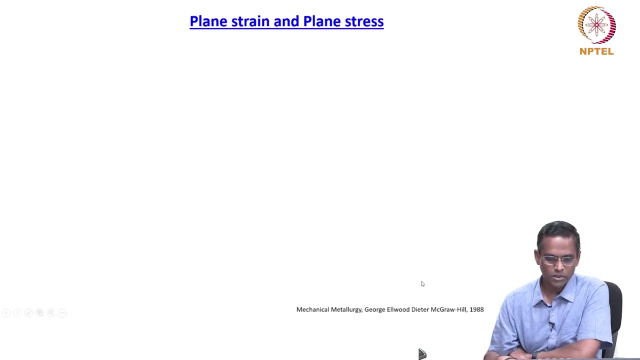 in fracture problems and fracture mechanics, for example. look at some of the the stress and strain states and we will be using all these relations. So another important relationship is the expression relating Young's modulus, shear modulus and mu. is g is equal to E by 2 times 1 plus mu. it is all some standard relations. 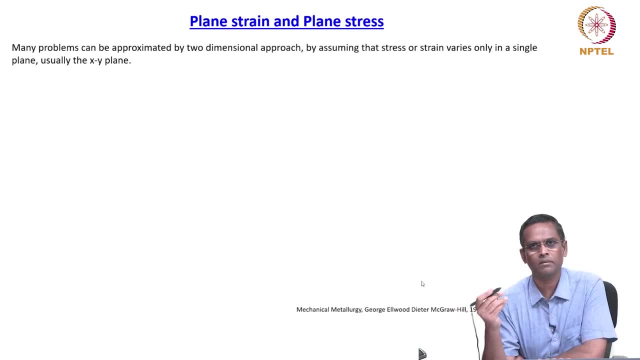 So now I am coming to another important topic, or I would say we are looking at fundamentals. So I am introducing another terminologies: plain strain and plain stress. So far we have looked at a strain in one dimension, strain in two dimensions, strain in three dimensions, strain in 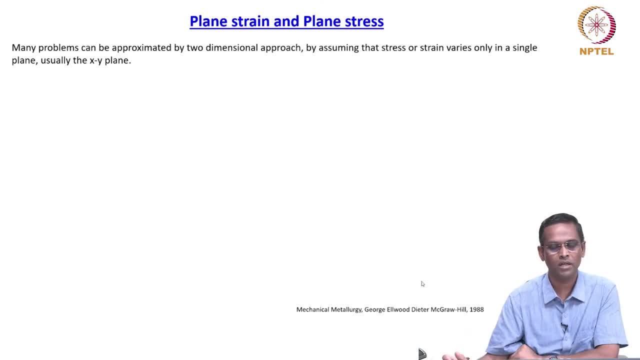 three dimensions: stress in one dimension, stress in three dimensions, but we did not talk about a plain strain or a plain stress. So the question is: why do we do that? The problem is, most of the engineering problems are in a practical, in a practical situations becomes. too complex. So if you make it a three, a three dimensional problem and reduce it to what? if you reduce one dimension, the mathematical treatment can be a simpler you can try to solve completely. that is the primary reason. So the many problems can be approximated by two dimensional approach. 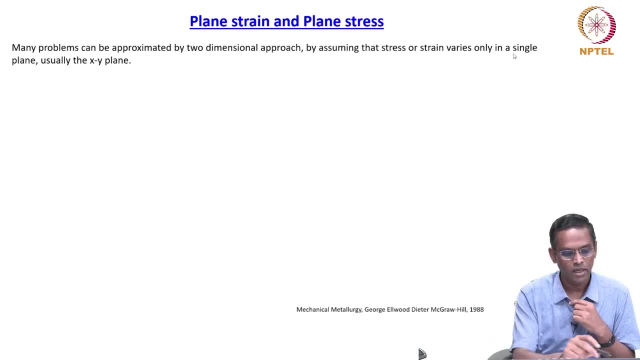 by assuming that the stress or the strain varies only in a single plane, usually an x- y plane. There are two ways to create such approximations. by assuming that the force normal to the plane is 0. The plane strain. this is called plane strain assumption. If you assume that the force normal, 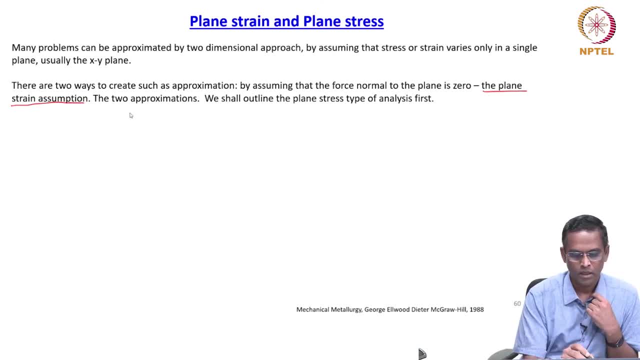 to the plane is 0, this is plane strain assumption, The two approximations. we shall continue or we shall outline the plane stress type of analysis. first We simply take equation of generalized Hooke's law and put: sigma x is equal to 0, then we 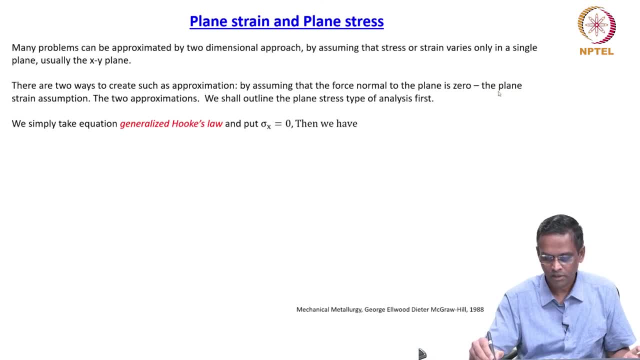 we have just developed three equations for as a generalized Hooke's law where you put simply sigma x equal to 0, then we get this equations. So I have shown three equations and if you just plug in sigma x equal to 0, then you will have this: 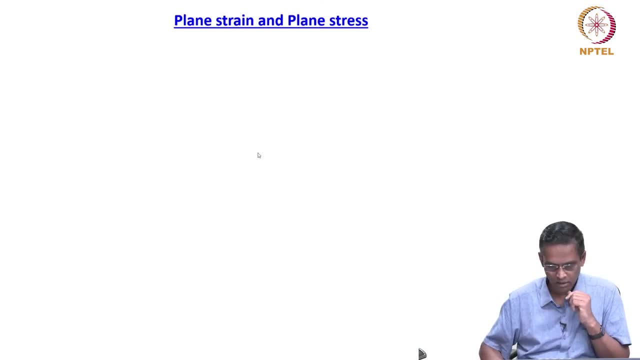 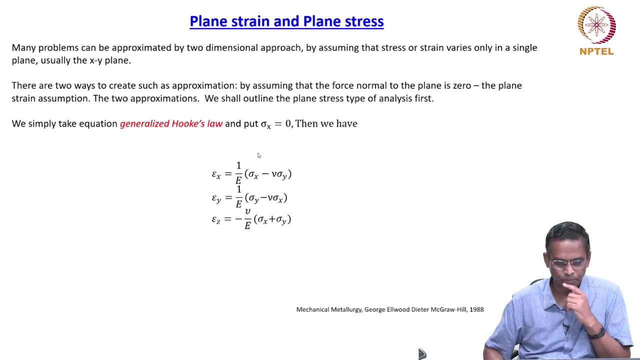 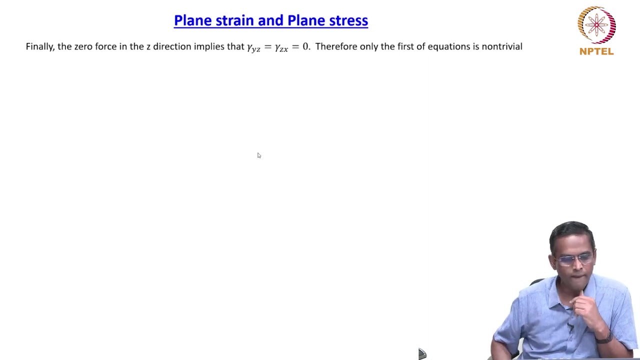 set of equation. this is valid for- sorry, this is a planes stress type Equation. So this is exactly for shear strain. So zero force in the z direction implies these two components become 0. Therefore, only the first of the two equation is: 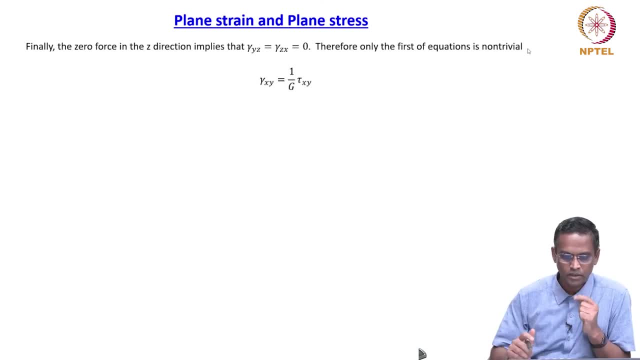 non-trivial. So this is a condition for the plane strain problems. Sorry, plane stress problems, These two equations. what we have shown is a plane stress formation For a plane strain analysis is a little more complex. by putting epsilon, z is equal to 0.. The Hooke's law gives an expression for sigma x. 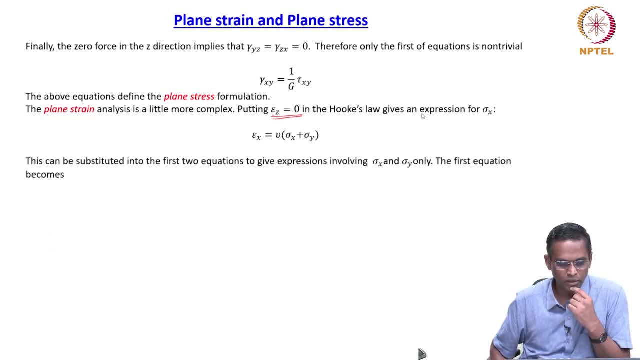 is this, and this can be substituted in the first two equations of the generalized Hooke's law Involving sigma x and sigma y. only Then this equation becomes like this. So it looks a little complex, but actually it is not. if you just plug in this: values there. 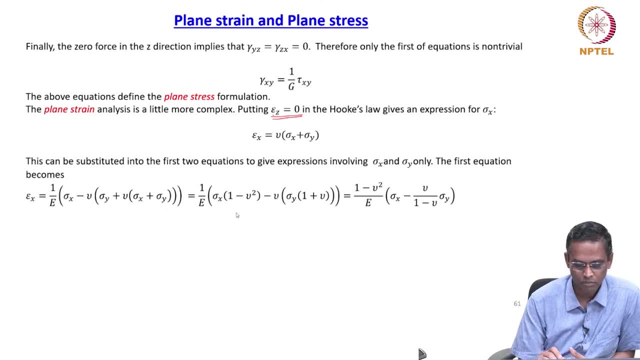 Then you yourself will find out that this is simple to manipulate. but what is important is the new terms which will emerge. that is what you have to focus by. just that is why this plane strain analysis is been complex. By this we can do hip hebcaach, because we know that likes and 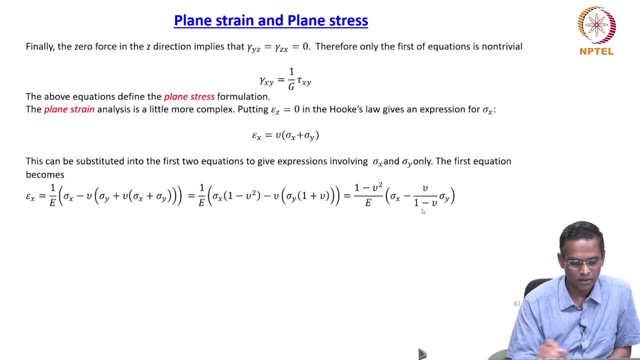 but you can just appreciate by looking at this expressions. So just plug in this assumptions into this and then you will get finally this expression: epsilon x equal to 1 minus nu, square by E times sigma x minus nu, by 1 minus nu times sigma y. We can simplify this. 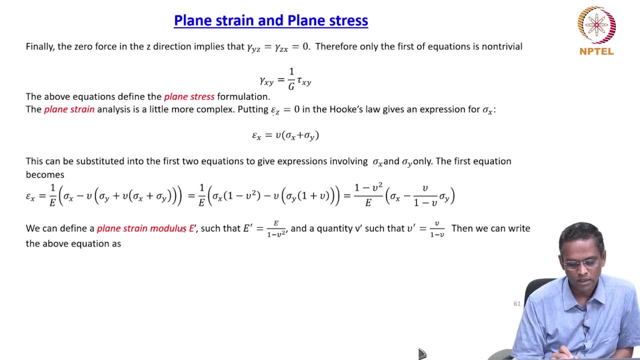 we can define a new parameter called the plane strain modulus, that is E prime. that is, E prime is equal to E divided by 1 minus nu prime square, and a quantity nu prime, such as nu prime, is equal to nu by 1 minus nu. 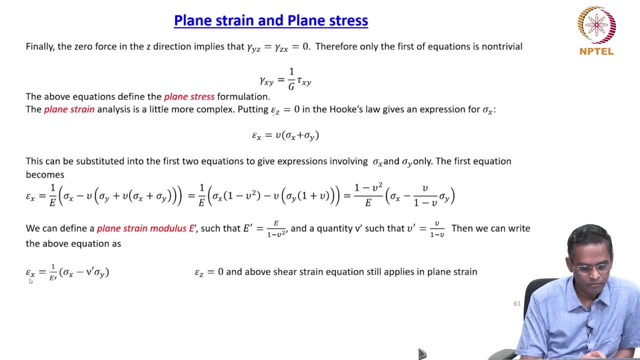 Then we can write the above equation: as epsilon x is equal to 1 by E prime times sigma x minus nu prime sigma y, Sigma z is equal to 0 and the above shear strain equation still applies in a plane strain. So why I have brought this particular? 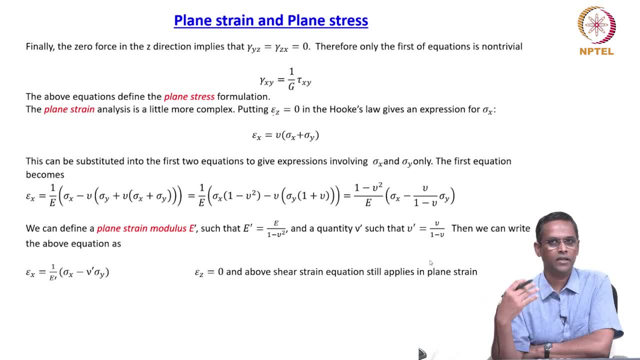 derivation is because you will see that wherever the problems are described, suddenly you will see that you know this: 1 by 1 minus nu term comes, or 1 by 1 minus nu square terms will come In most of mechanics problems, but people just do not pay attention to this. See, it will come how So. 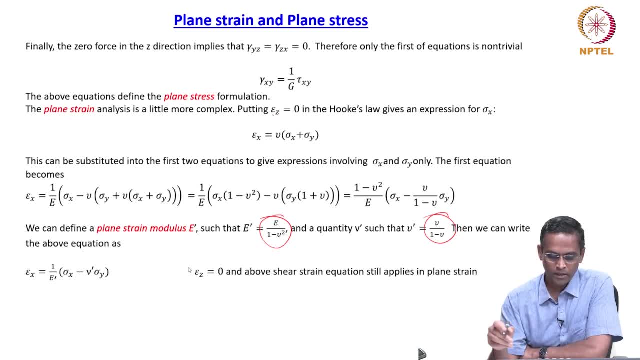 this is how it will be. If you just work it out, then you know that. okay, so that is because we are manipulating the Young's modulus. The Young's modulus will have some different effect in the plane strain condition and that is why we are doing this. So that kind of alertness will be useful. 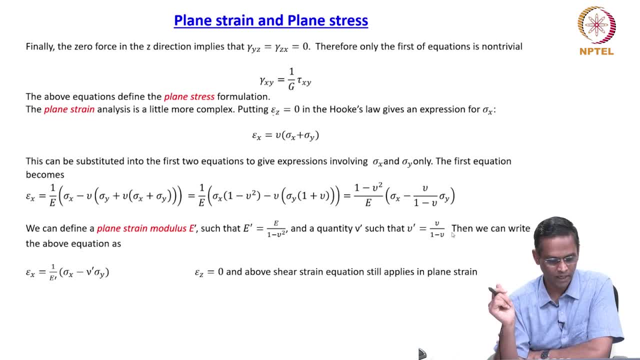 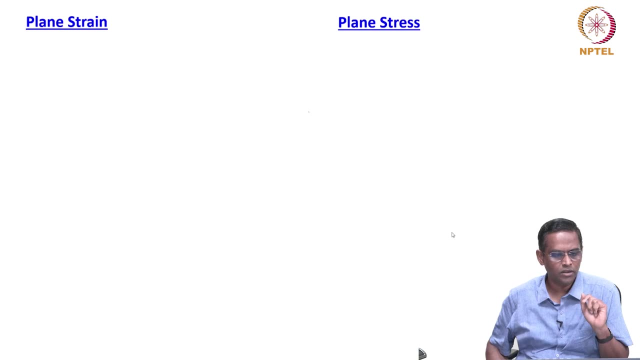 Instead of simply looking at the expression, what is given in the textbook, you can just derive by our self and then see, and then get familiar with the terms. That is the purpose of this slide. Otherwise there is no significance here. So now in general, in a plane strain. 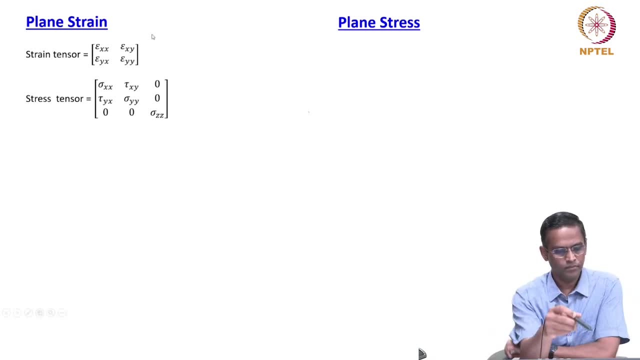 you can write strain tensor like this: epsilon xx, epsilon yy and epsilon xy and normal strain and the shear strain, normal stress and shear stress. So please remember, in a plane strain condition, strain tensor is 2 by 2 matrix. For a plane strain condition, stress tensor is 3 by 3 matrix. 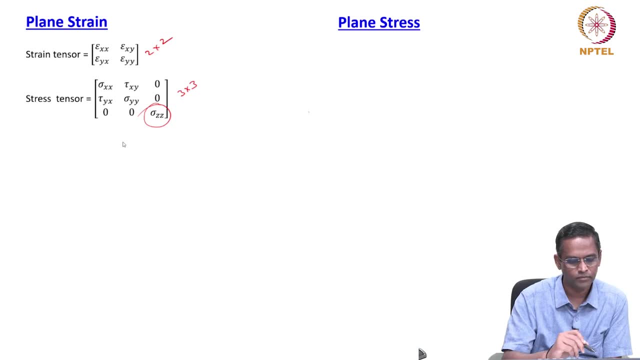 Okay, so you get, this is not 0. So this is very important. We will see when we discuss in a fracture mechanics concerts. So it will be. you know, dimple formation in a crack tip when we when very high stresses at the crack tip. So I will show some examples. when this kind of examples practical 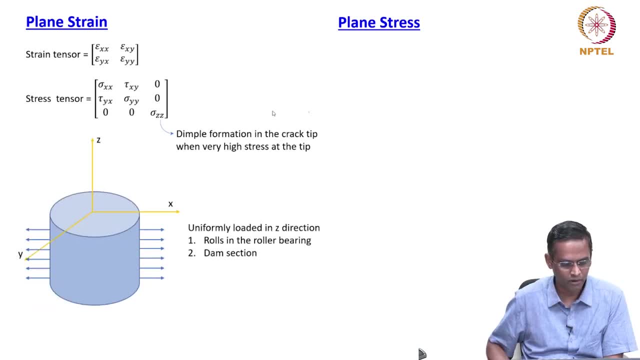 examples when we discuss that subject. So this is a schematic for plane strain and real-time examples are rolls in the roller bearings and dam section. they are all considered to be plane strain condition. And what is plane stress? This is: this is schematic for a plane stress. 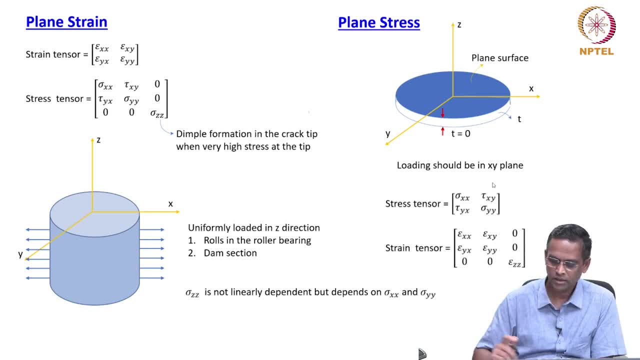 Loading should be only in xy plane and this is a stress tensor and this is a strain tensor. okay, So the stress tensor, again it is for a plane stress, it is 2 by 2 matrix, but not the strain tensor. Strain tensor is 3 by 3.. So epsilon z z is not 0. So 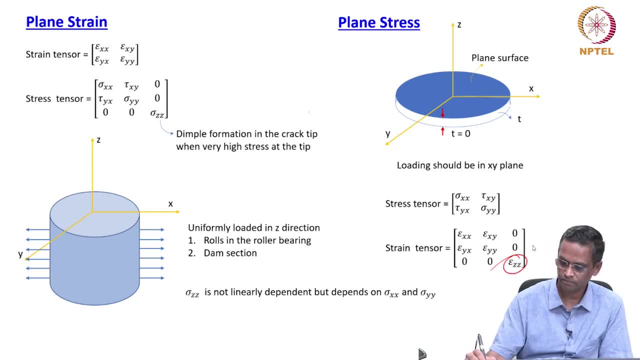 this is again a very important point to remember. okay, So that is that these are all the introduction to this, stress-strain relations. I just want to review, and these are all, some of the fundamentals given in all the textbooks, but some of the subtle. 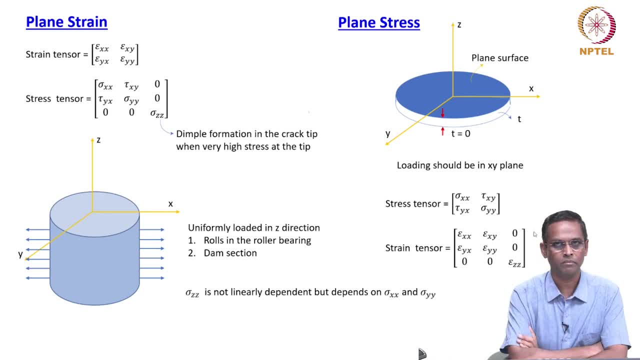 differences, small, small details. people do not pay attention, then they struggle to get the idea. So that is idea I. that is why I just wanted to review this, though it is simple, So I will from. I will stop here today. See, one important point is I have flipped the slides pretty fast. 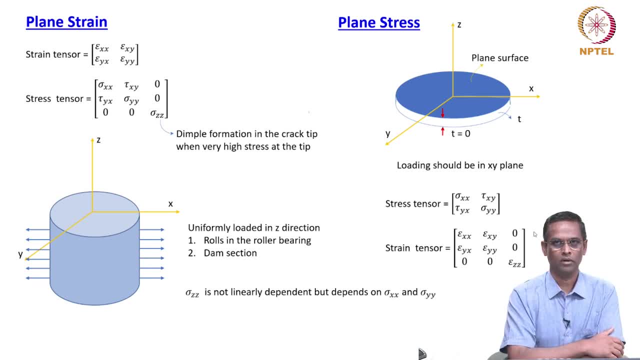 and if you start writing on the blackboard, it is always good, okay, Especially when I write too many equations on a slide, and that too, if you just flip it through just by reading, it is very difficult to follow. So what I, what I request all of you to do, is, if you look at any of the expressions, you 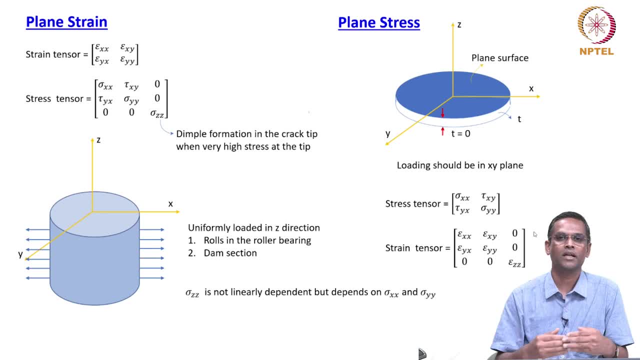 try to write. first you look at the video and then try to write of your own in your notes and then see whether you are getting. you are getting this expression of your own derivation: So small, small relations. but then you have to practice that. 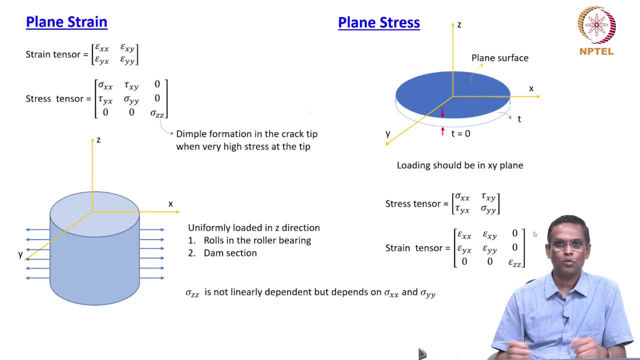 there is no other goal right. Even if I try to do it on the blackboard- and it will be, it will take lot of time, but these are these important things you have to do And if you have any difficulties, you can always write to us. and when we have the interaction,